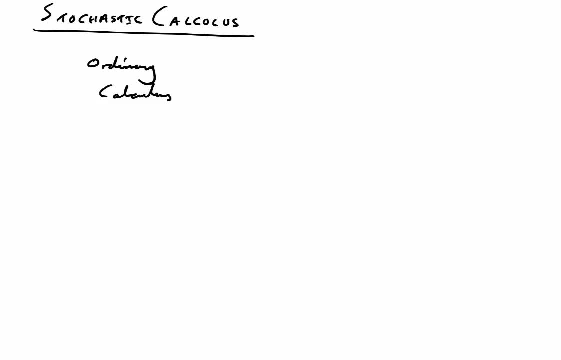 find the gradient of a straight line. you know we can't find the gradient of this jagged line. you know it doesn't matter, It doesn't, it never becomes straight. okay, So really, this is where stochastic calculus comes in. 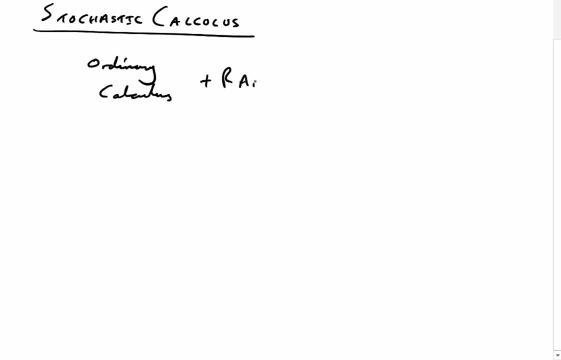 and it's just basically ordinary calculus, okay, but it includes the randomness, the randomness element, okay. So let me kind of show you what I mean by that. Well, kind of you know, you've already seen this before, so I'll show you using the example that we had before. So here we go. 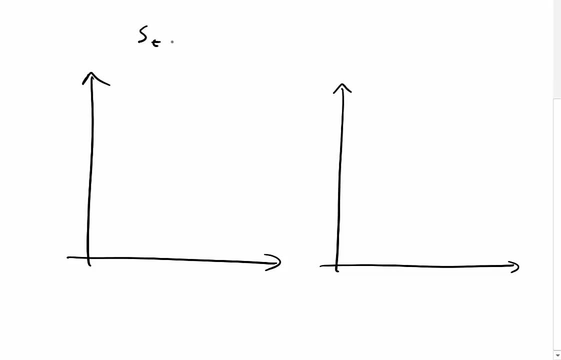 okay, Now if we had you know, the share price is given by the initial share price. so the share price at a time t is given by the initial share price, times by some growth rate and that's an exponential growth rate. 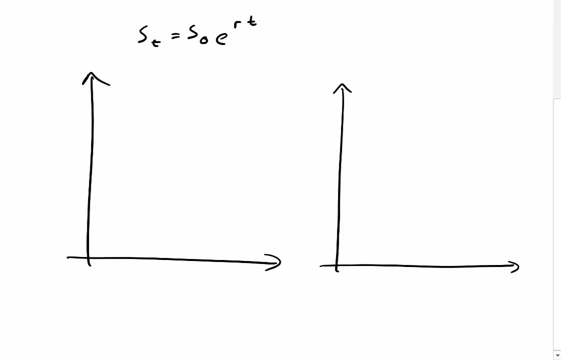 okay, which changes over time, and the rate is given by r okay. So we have st equals s naught e to the r t. So if this is st okay and this is t all right, then we start. we start at s naught. 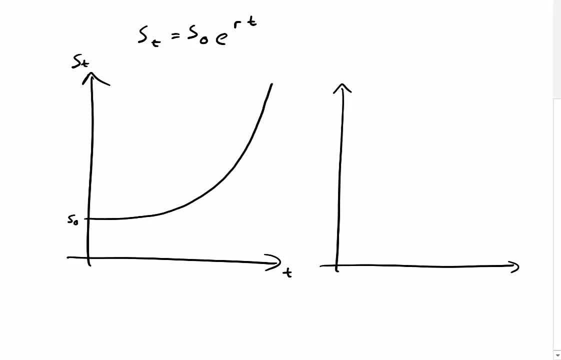 okay, and we follow this kind of exponential growth and we can differentiate that using normal calculus. we can differentiate that using normal calculus. okay, We can basically say that the derivative of our share price with respect to t- okay, will be given by. well, what's basically? 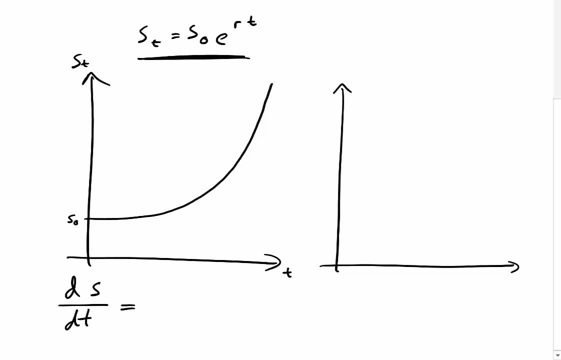 the derivative of this. Well, the derivative of this is going to be: you know we have s naught. okay, e to the r? t, it's an exponential function, so it's just going to be the, you know s naught is. 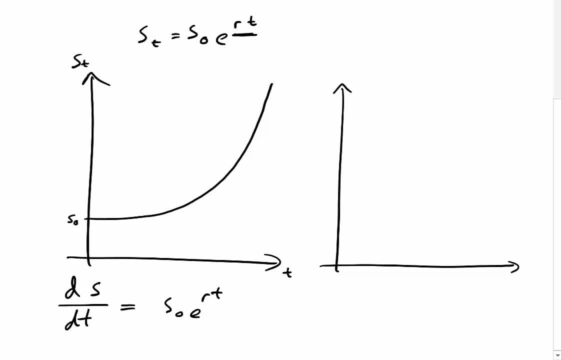 just a constant. okay, so it's just going to be the derivative of r t multiplied by all of this. so the derivative of r t with respect to t is going to be: what's it going to be? it's going to be r. 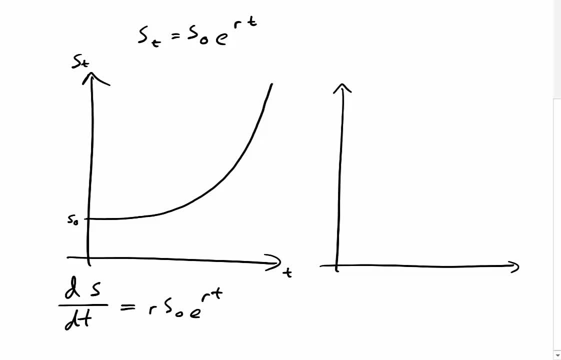 so we end up with r s naught e to the r t: Yeah, are you happy that that is just the derivative of that? Okay, basically, what we're asking is the derivative. say, for example, you have the derivative with respect to x, of e to the function of x, okay, or even just a constant times e to the. 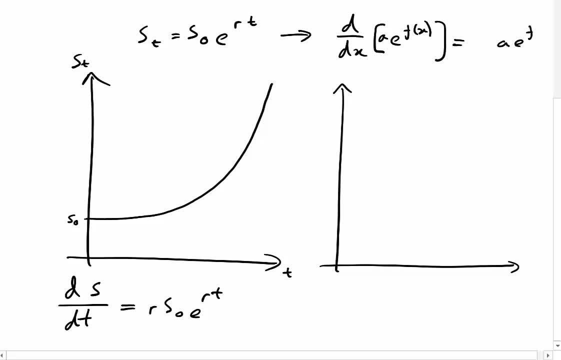 function of x. well, that's just going to be the same thing multiplied by the derivative of this power. yeah, so the derivative of that function. so that's all that's going on there. so that's all I'm doing down here. So basically, I can say that you know the derivative of my share price. 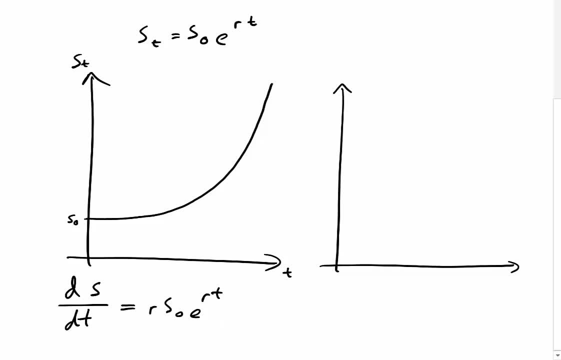 is r? e to the s naught e to the r? t. but look, look, what s naught e to the r? t is. that is that there, which is s t. so I can just rewrite this as r times my share price, so my rate times. 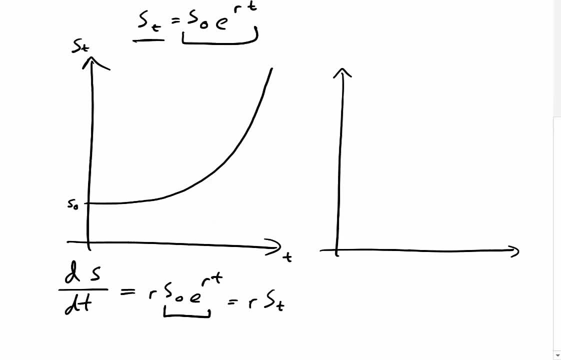 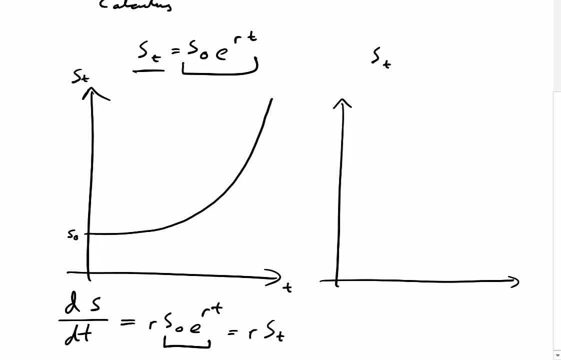 my share price okay and I, yeah, okay. so this is what kind of what I would do using normal calculus. but of course I've said that now you know, a share price normally models not this kind of growth rate. I mean, this is, this is kind of a good model for kind of showing how the share 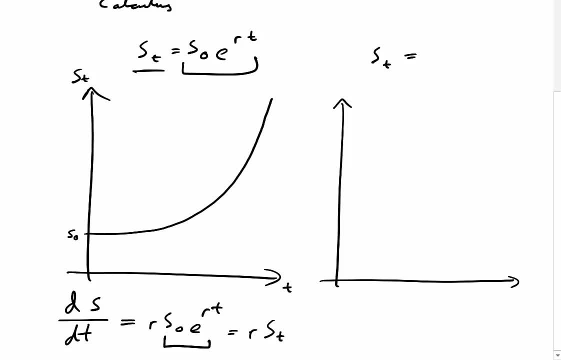 price changes. it's an exponential growth rate, right, but it's actually it's this thing. it's s naught e to the r? t, okay, but we have to include Brownian motion into it. so, in other words, you know, this is still s? t against t okay, and it follows the. 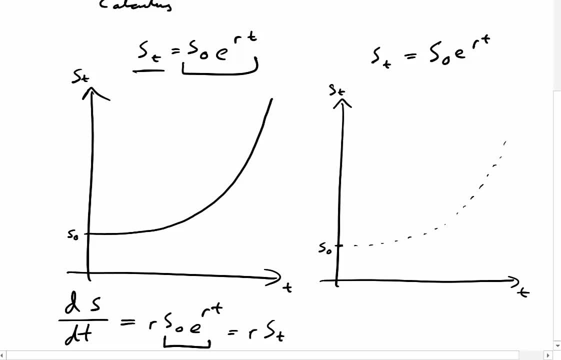 same kind of shape follows the same kind of shape as that, but this time we have Brownian motion added and we say that it's Brownian motion. okay, we can have any constant times, Brownian motion, and actually I've talked about that constant beta before with the Brownian motion. 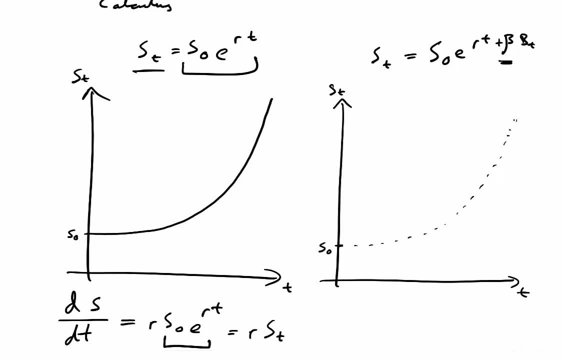 it's really, really difficult to find. actually, there's whole sections of the industry, whole divisions of the industry, that are devoted to trying to find out what that beta is. okay, but it's beyond the scope of the data, this course. I just want you to be aware of that, okay? so, essentially what this? 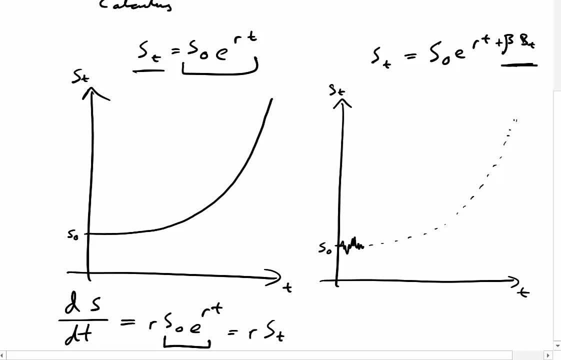 what this term does. it just accounts for the randomness. so basically, we have this kind of random pattern and this is kind of your familiar Brownian motion that's happening okay. so here we go. it's going to look like that. so this is what the beta t. 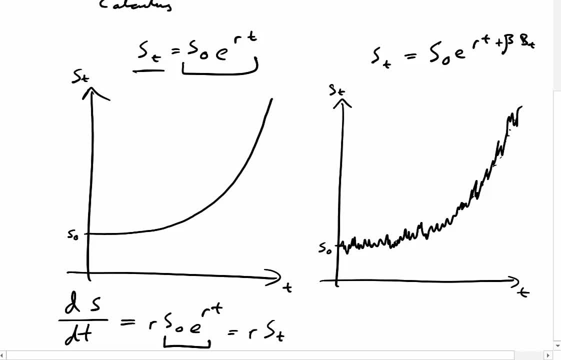 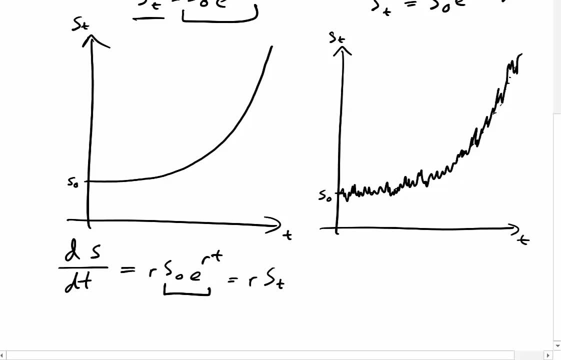 term is doing. it's kind of adding the Brownian motion, if you like. well, obviously, trying to differentiate this Brownian motion, okay- is going to be much more difficult and therefore this is where stochastic calculus comes in, okay. so it's kind of it's random, but it's not too random. 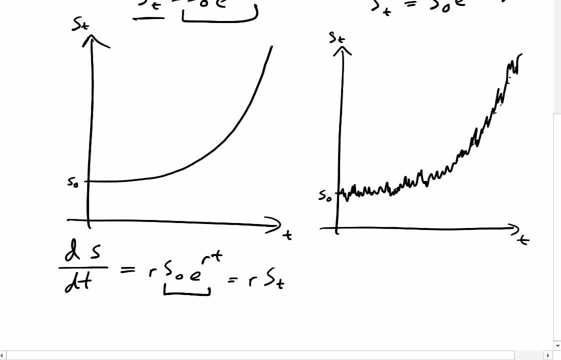 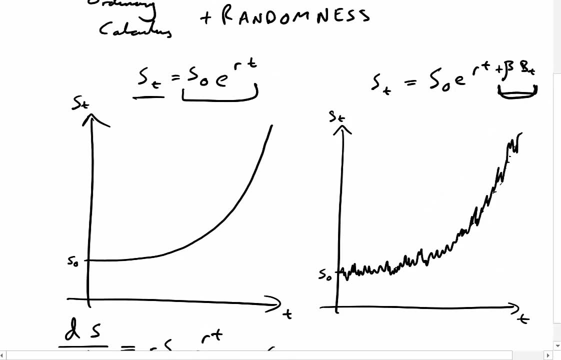 it does still follow some kind of pattern which allows us to use stochastic- you know stochastic calculus. so basically, what I'm talking about is this thing here. okay, I've said it's random. well, it is random, but it's randomness, that is. 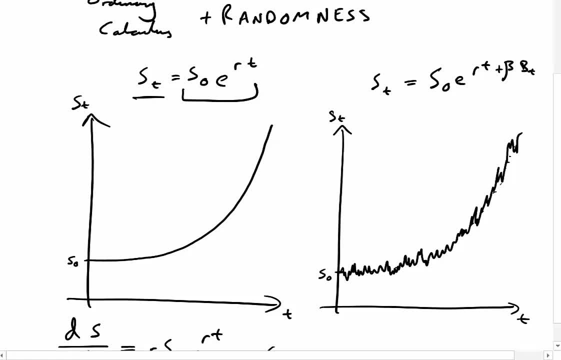 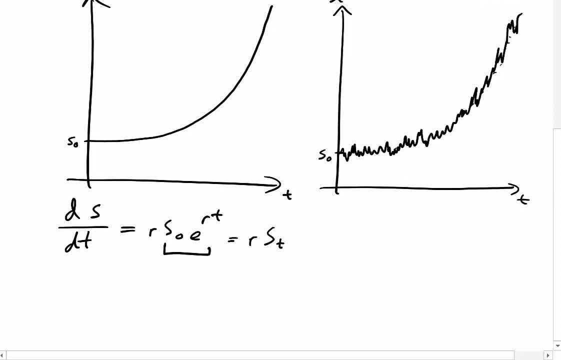 that comes from something within you know it's how the share price moves effectively, so it does have some kind of distribution that can be used using. that can be found using you know that can be found using stochastic calculus. so in other words now what I'm saying. 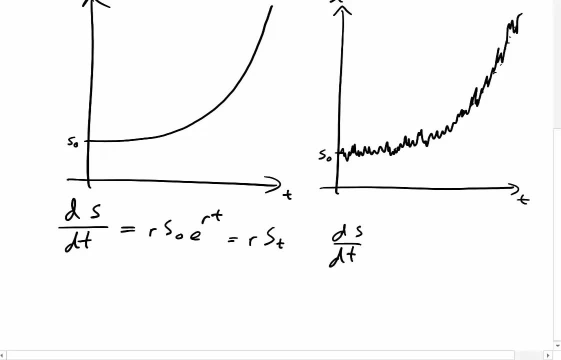 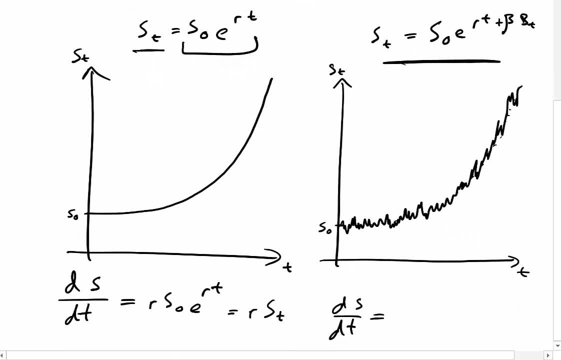 up here. let's see if we can get that in frame. there we go. then this will be equal to this, will be equal to the same thing that we had before. so r or no, actually wait if I try and differentiate. 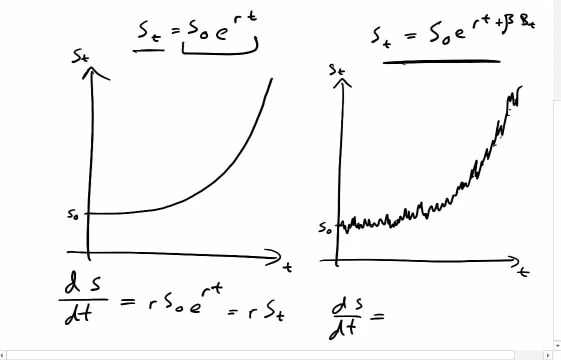 it using ordinary calculus. right, I'm going to have to. I'm going to have to use. I'm going to have to. if I try and differentiate using ordinary calculus, as it turns out it doesn't have any meaning, but let's try and do it anyway. so say, for example, I'm going to have to use, I'm going 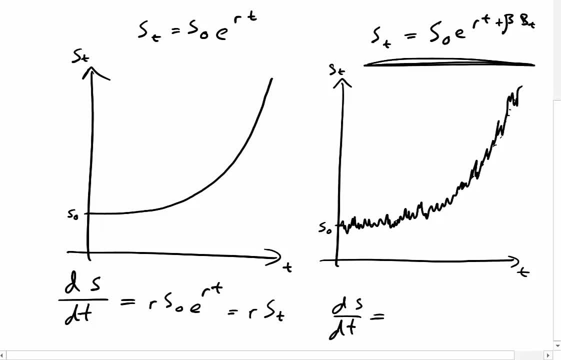 to have to use. I'm going to have to do it anyway. so say, for example, if I could differentiate this using ordinary calculus, what would I end up with? well, it would be, you know, it would be s naught. it would be. it would be, it would be, you know. it's basically. what I'm saying is the 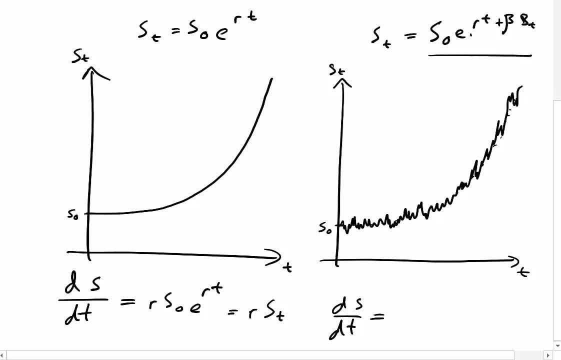 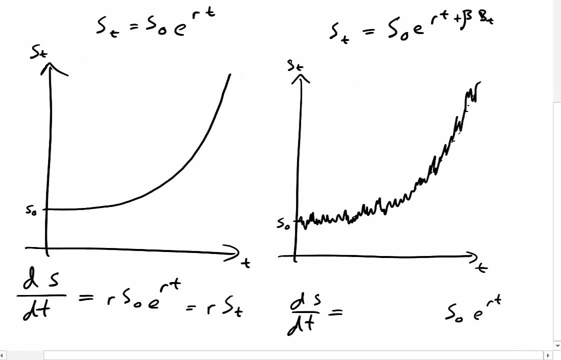 derivative. it's this multiplied by the derivative of this power. so, in other words, what I'm saying is it's going to be s naught e to the r t plus beta, b t. okay, multiplied by the derivative, multiplied by the derivative of this power, okay. 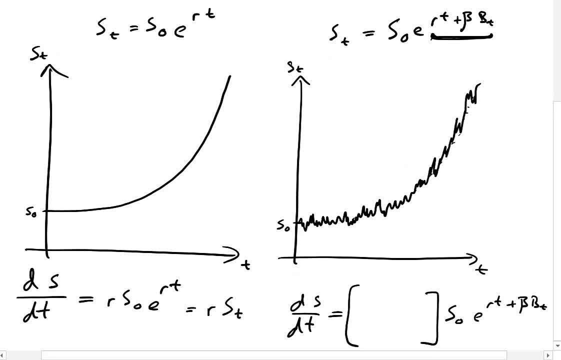 multiplied by the derivative of this power. so the derivative of this power would be r? t. so the derivative of r? t would be r. okay, plus plus the derivative of this beta b t. yeah, so this beta b t derivative of that with respect to t, that's going to be. 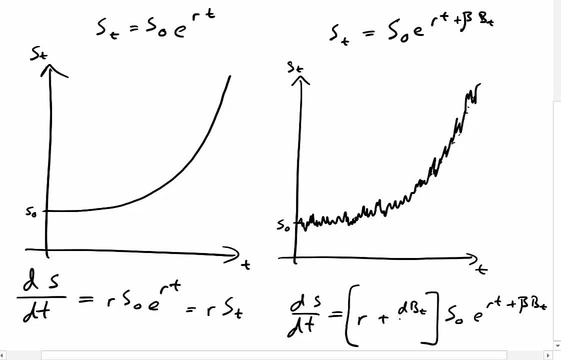 what's it going to be? it's going to be d b t derivative of b t with respect to time. okay, multiplied by beta, is that right? yeah, multiplied by beta. so let's see if I can squeeze a beta in. 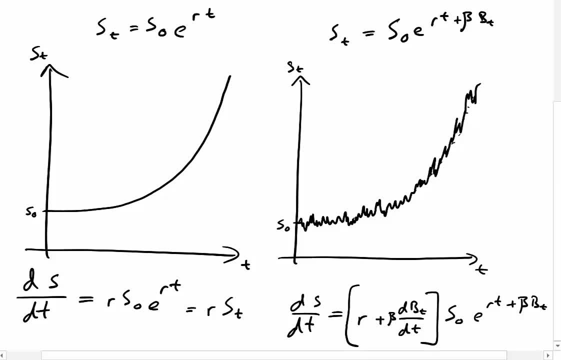 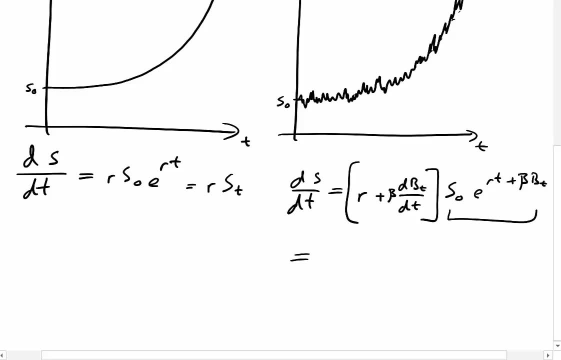 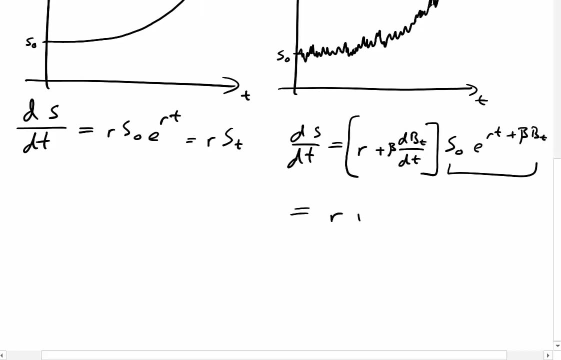 there multiplied by beta. so add those two things together. okay, fair enough, let's now try. and well, that's basically what this is saying. now is this: is this here? you're happy? this is just my s? t. yeah, it's just my s? t, it's just that, okay. so this is now r plus beta: d b t by d t. 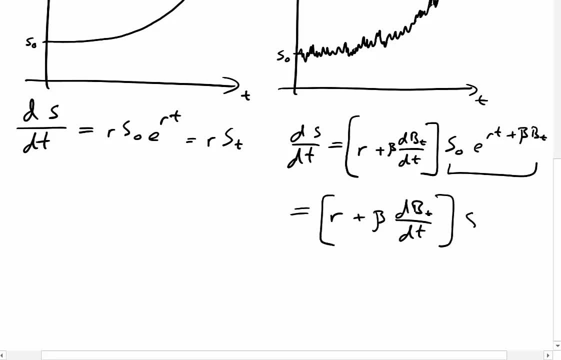 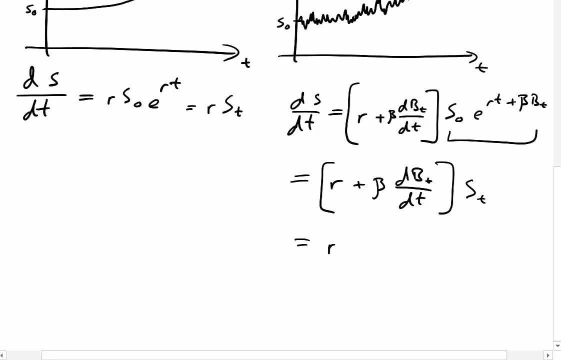 so the derivative of Brownian motion multiplied by my share price s t okay. so this is what. this is what we end up with, and actually I could probably expand that out. so r s t plus beta d b t by d t. 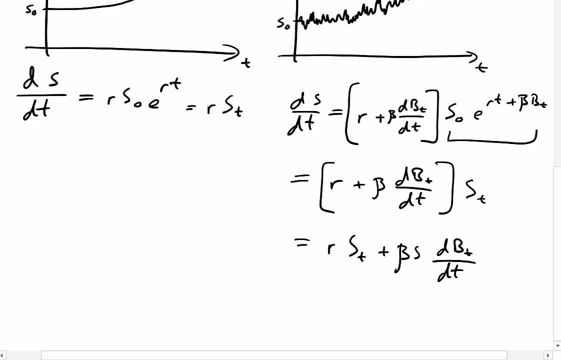 and I'm just going to stick the s? t at the front there. so s t there. so this is what I end up with. but basically this is where the problem comes in, because what is the derivative of Brownian motion? well, that's where the problem comes. that's where the problem comes. okay, now I'm just going to 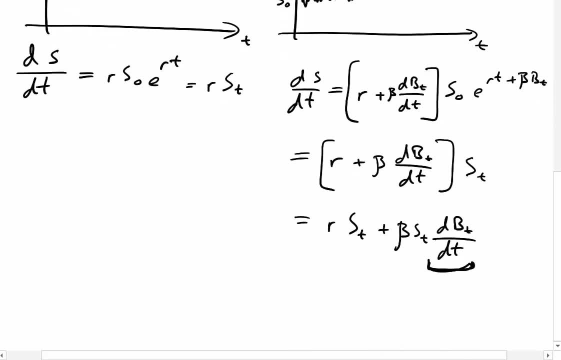 introduce something new now so it doesn't come as too much of a shock later on- or I don't mean a shock, but I just mean so it's not brand new later on. you know, at least you're familiar with it- I'm going to introduce: 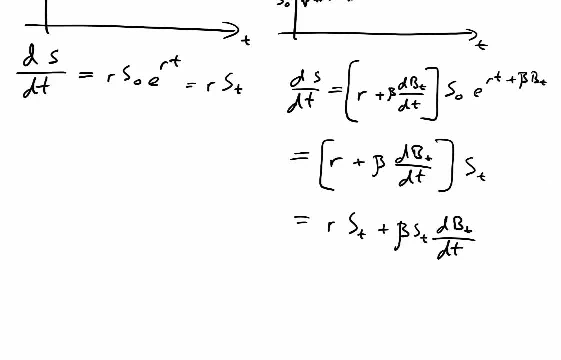 this idea of what's known as differential form. well, differential form is basically rewriting this thing, rewriting this thing. so it's just well, let me show you what it is and then, kind of hopefully, you can see what's happening. so right, d s, d s? t. effectively, this is. 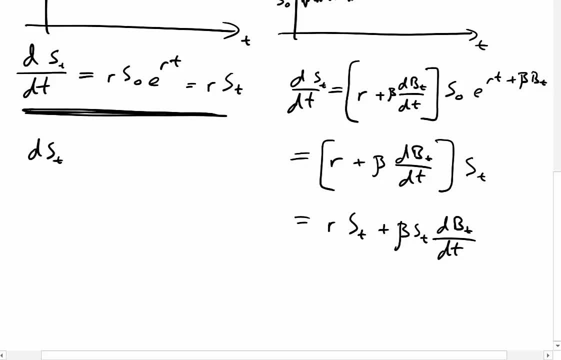 you should just get the t in there. d s t with respect to t. so I'm just going to rewrite it out. first of all, equals r s t, just equal to that thing, right? well, what differential form is is? it's basically writing. 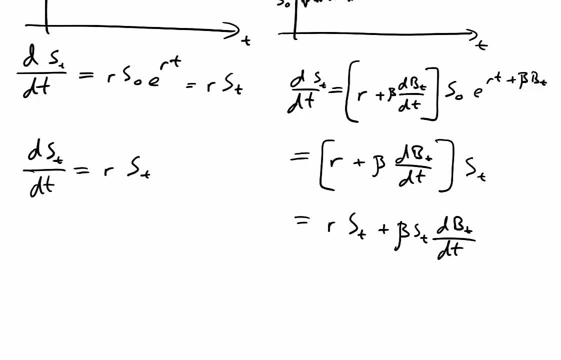 it in such a way. it's a bit like when we're doing separation of variables for ODEs, if you, if you kind of go back and watch my ODEs variables. basically, what we try and do is we treat this as a fraction, we treat this as a fraction and we get everything involving 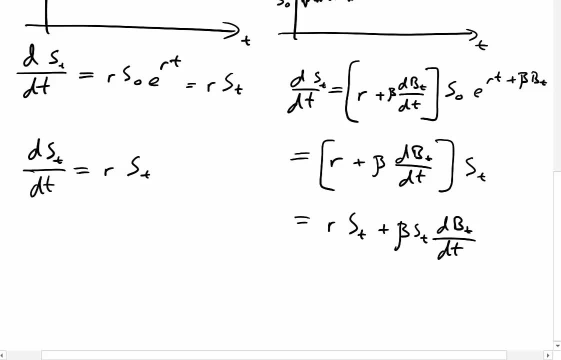 and we just basically multiply through by dt. so in other words, it makes the integration. you know, we can kind of integrate it. then it's a bit like separation of variables. in other words, what I'm saying is that we just have d s t still here by dt. 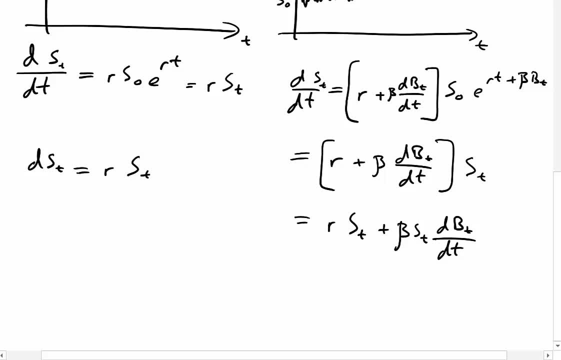 if I just multiply through by this dt effectively and write it like this, this is what's known as differential form, because it kind of makes you know. hopefully you can see that you know it kind of links to it, kind of links to the integration. 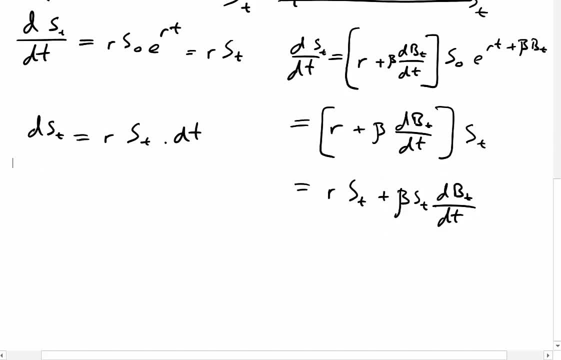 okay, like that. okay, so now let's try and get this, this thing here, into differential form. so we end up with: this is the differential form for the ordinary calculus case. this is: d s t by dt equals r s t plus beta s t times the derivative of Brownian. 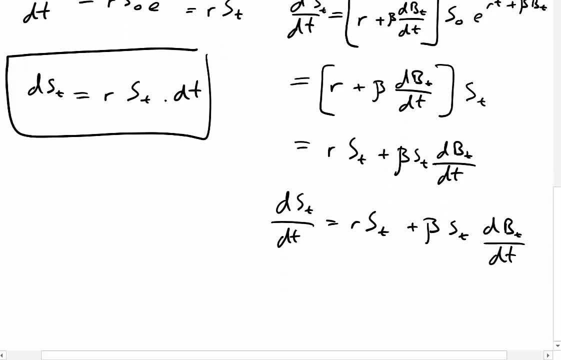 motion with respect to time. okay, so that implies that therefore, we end up with d s t. so just multiply through by dt is equal to r s, t, dt plus beta s t, d, b, t over dt multiplied by dt. okay, so are you happy that those two dt's just effectively cancel out? just cancel out. 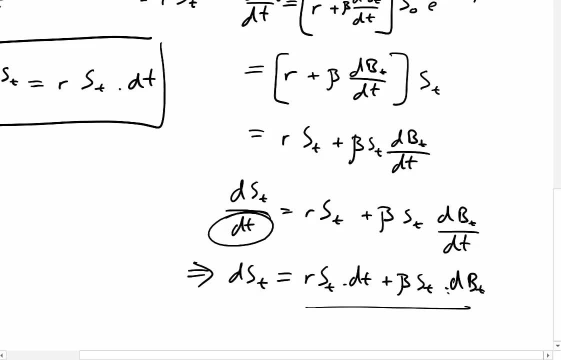 so then this is what we're effectively left with, but again, we've still got this. problem is: what is the derivative of d beta by dt? and this is actually useful because we can use something known as an Ito's lemma that looks at this okay. 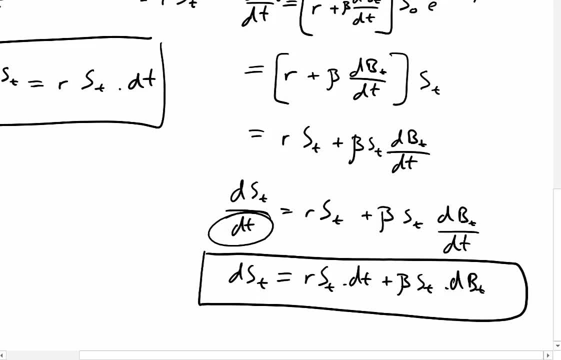 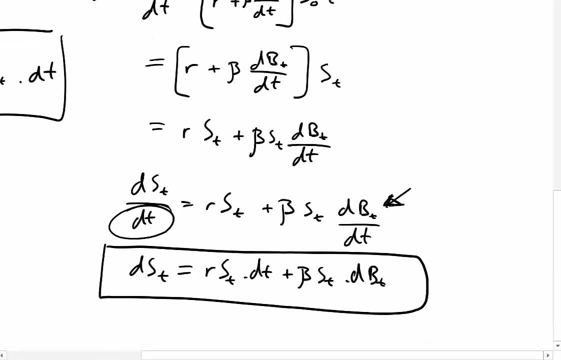 so we'll look at this in a little bit more detail in just a second. okay, but in actual fact, because we don't know what the derivative of this is, then we can't. we can't actually use differential calculus. so what I've just written down here, you know what I've written down here. 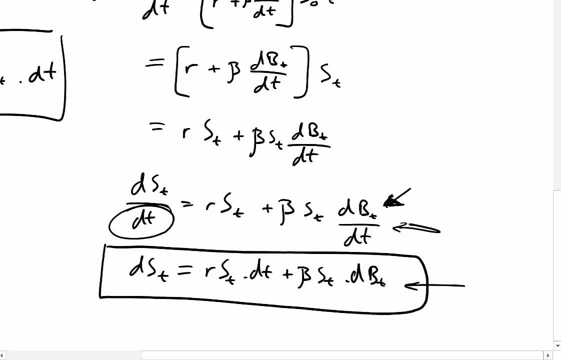 or what I've written down here. they're the same thing. what I've written down there doesn't actually have a lot of meaning. doesn't have a lot of meaning in the kind of ordinary calculus sense, because we don't know what the derivative of Brownian motion is or we can't differentiate. 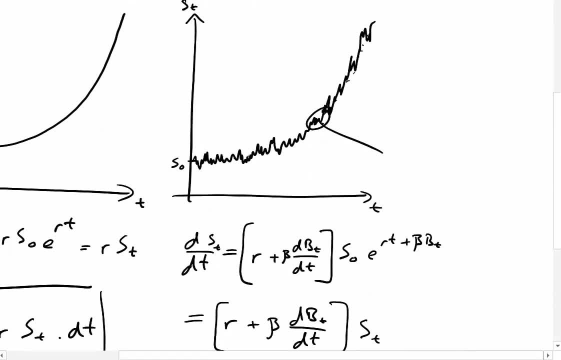 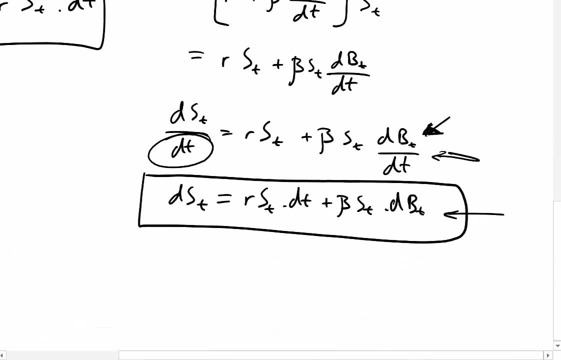 Brownian motion because of this thing. basically, if we zoom in into it, if we zoom in on it, you know infinite amount of times it's still going to be jagged. so we can't differentiate jagged jaggedness. it doesn't go straight. so, yeah, hopefully that. 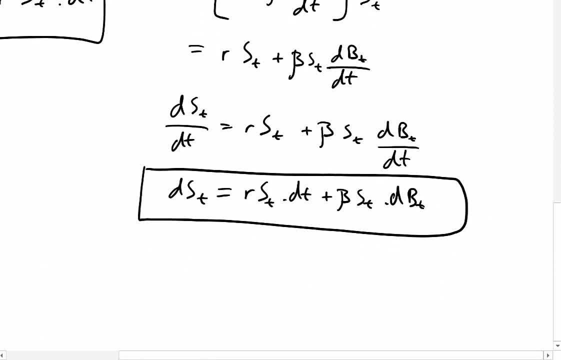 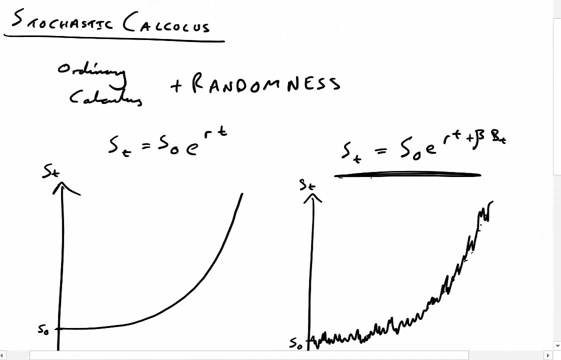 makes a bit of sense. but essentially, yeah, so I've introduced. now, just in this term, I've introduced, I've introduced. you know the difference between ordinary calculus and you know the reason why we want to use stochastic calculus. hopefully that's kind of clear in your 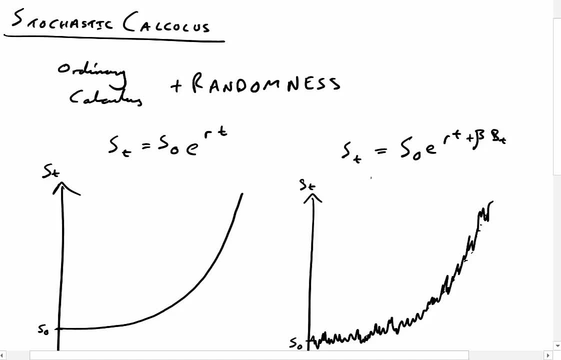 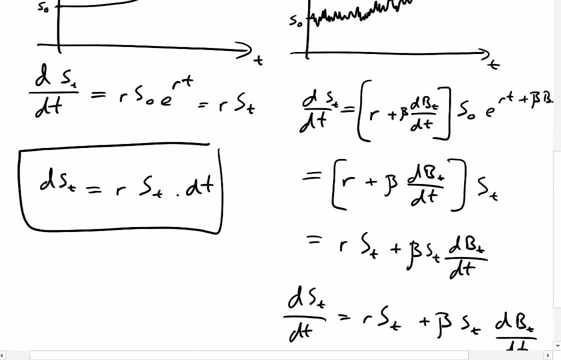 head. it's because of this Brownian motion, okay, and I've kind of hopefully shown you that you know how this, these two things, link together and what we would do if we were differentiating that thing. that's nice and easy, we can do that, but this thing doesn't have a lot of meaning because, because of 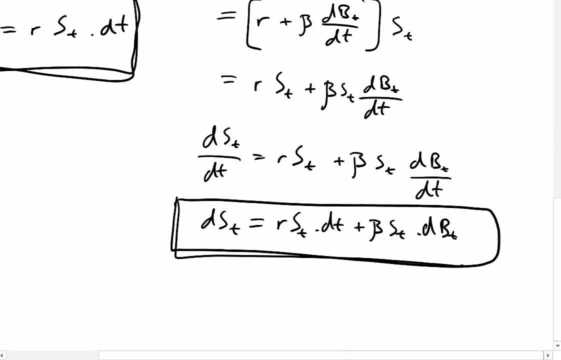 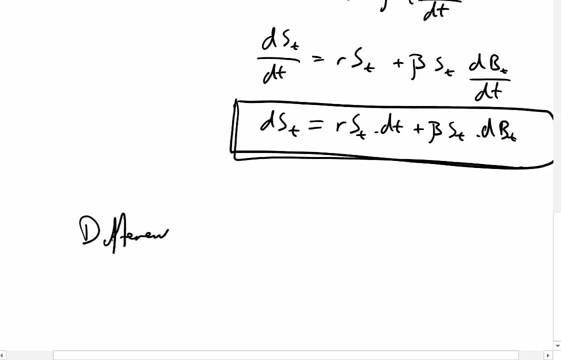 this term here the derivative of Brownian motion, okay. so basically, what we're going to do, what we're going to do normally: normally, when we teach calculus, you teach differentiation first, okay. so when you're learning it on your A-level, you teach differentiation first, okay, and then from 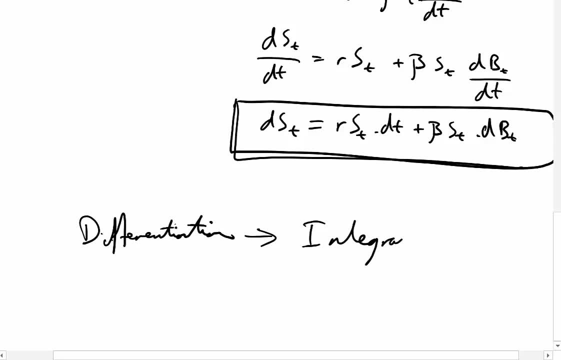 that you lead on to integration. okay, you lead on to integration. so you get the idea of differentiation first, okay. then from that you lead on to integration. you see that integration can either be treated as something totally different to differentiation- differentiation is finding the gradient, okay- whereas integration 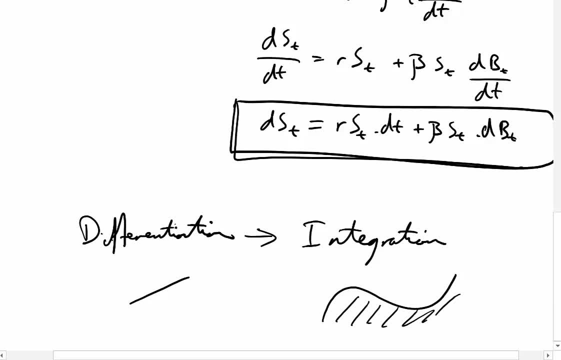 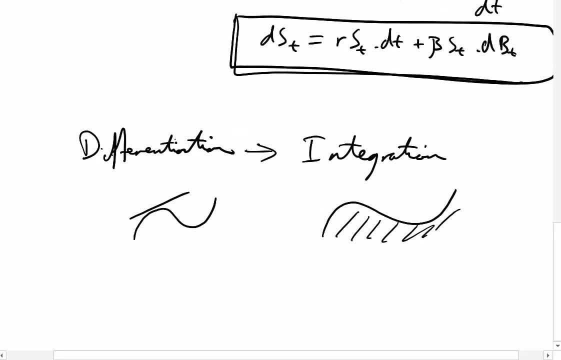 is finding the area underneath the curve, okay, differentiation is finding the gradient of a curve, right. so kind of you can see that they're two different things, but equally you can see that actually by the fundamental law of calculus or theorem of calculus that they are actually.